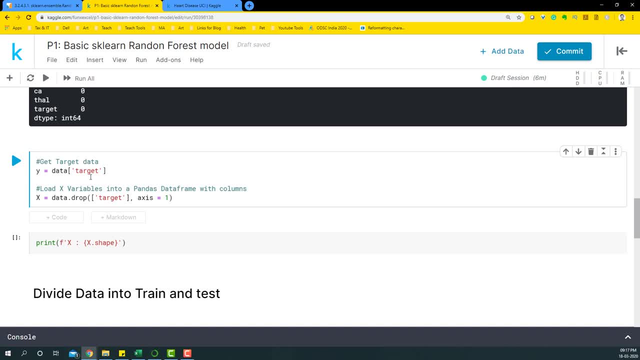 next step. Then what we will do is: now we will get the target data within y variable and from the data set. I am just going to take the target data. Whether a person has heart disease or no, this particular variable will be telling us Now. next we are going to load the x variables. drop just the target variables so that the 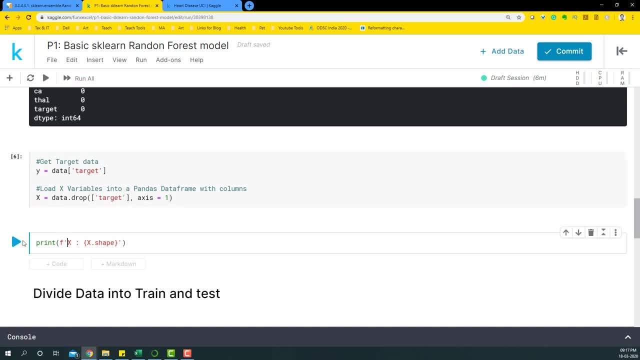 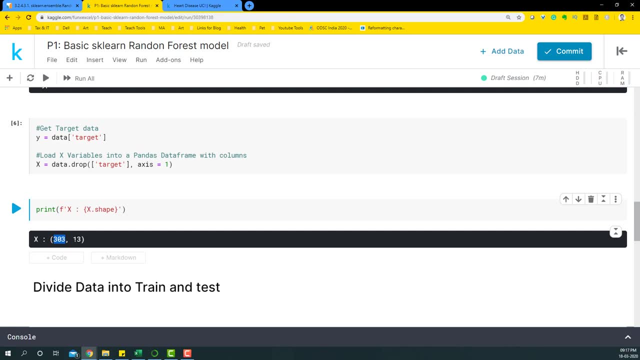 rest of the variables are going to be with you Now. if I run this and print the shape of x, The x variables, you will notice that there are 300 rows, 303 rows and 13 variables. Now, this is what our basic modeling setup is going to be looking like. 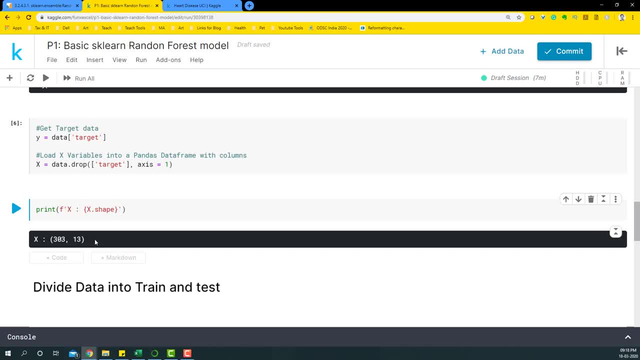 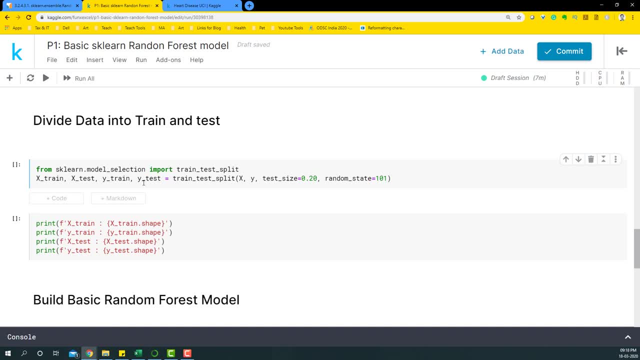 For the next steps. what we are going to do is we are going to divide the data into train and test. So for that we are going to take the sklearn model selection train test split method and divide our data set into 4 different data sets. Now, once I do the division, let's 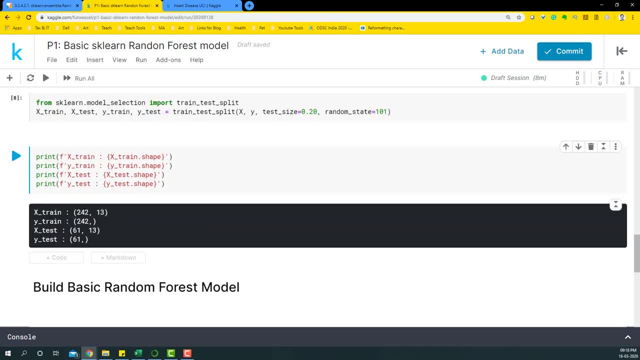 check out all of the data sets and their sizes. The x train data set will have 242 rows, which is roughly 80% of 303 rows, and 13 columns. The y train will be 242 rows, same as the x train, and it will only have one column, which. 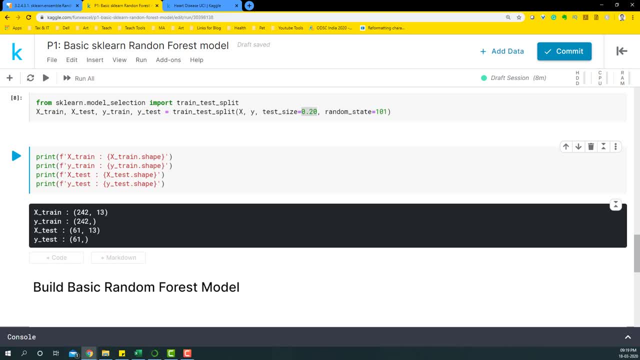 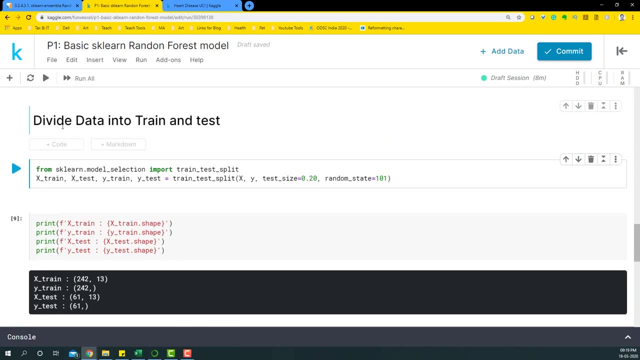 will be basically 0 or 1 the target variable. Similarly, we have x test and y test. They will have 61 rows, which is nothing but 20% of 303 approximately. Now we are going to take the x test and y test. They will have 61 rows, which is nothing. 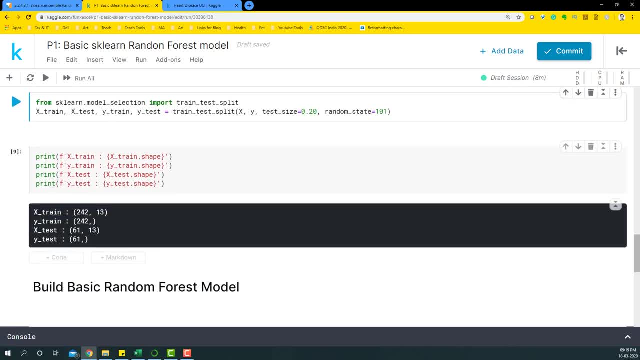 but 20% of 303 approximately. Now we are going to take the x test and y test. They will have 61 rows, which is nothing but 20% of 303 approximately, And obviously 13 columns, much like the x train data set. Also, it will have 61 values for. 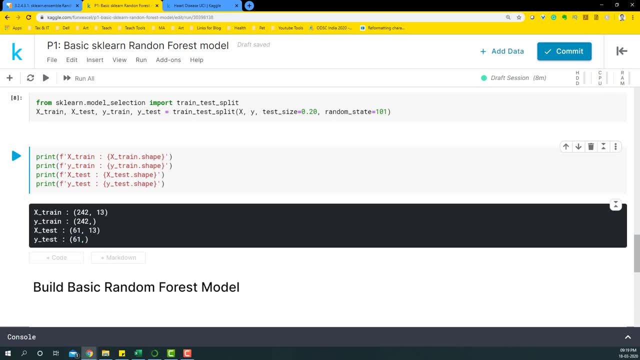 the y test, which will tell us whether that particular person has a heart disease or not. Now we are going to build the model on the train data set and then, on the test data set, we are going to check if that accuracy is holding good enough or not. 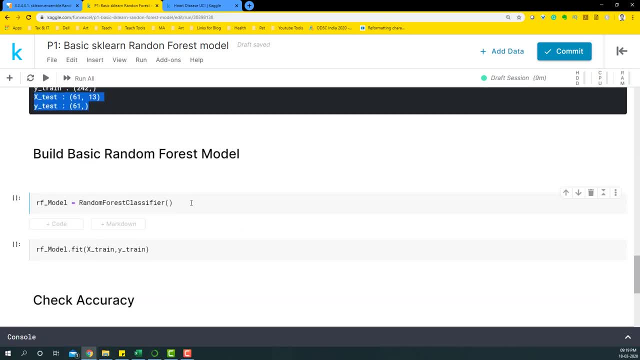 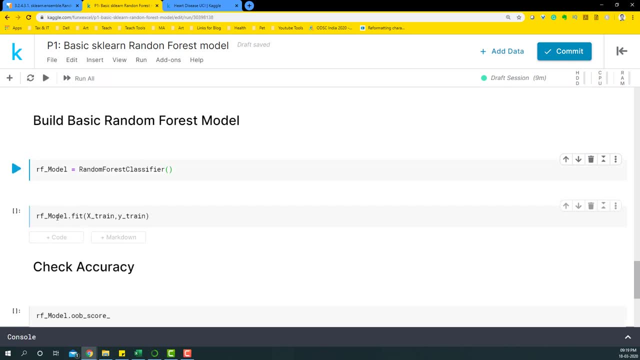 So let's build the first basic random forest model. First we are going to initiate an instance random forest classifier into RF model. now I've done that, I'm just going to fit the model RF model dot fit and this time I'm going to use the x train and y train data set to basically fit. 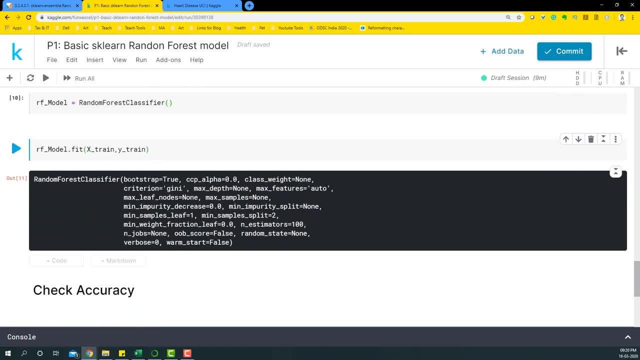 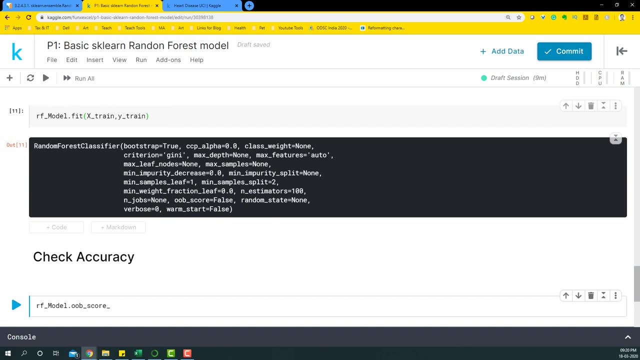 the model. now, once I fit the model, there are a lot of parameters random forest has and it has basically chosen some of the best ones that it could take. in random forest there are some parameters that are very helpful and then we can use parameter tuning there will be. 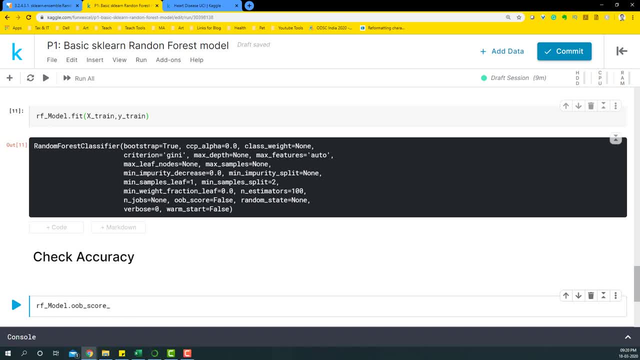 the criterion: max depth, max features, max leaf nodes, max samples, max impurity, max sample leaf, max sample leaf. split and estimators is one of the most important ones- njobs, OOBScore, and then random state and some other ones that are available right. so basically, there are a lot of parameters that we can. 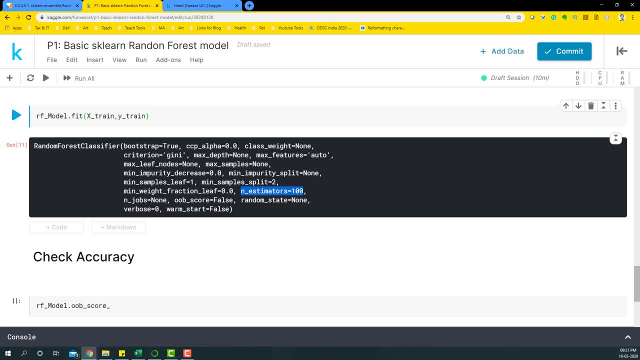 tune and we can use them for certain random forest much more than how we used them before. a lot of parameters that are very helpful and then we can use parameter tuning. they'll be the criteria: max depth, max features within random forest. in the next video we're going to be looking at the random forest model. 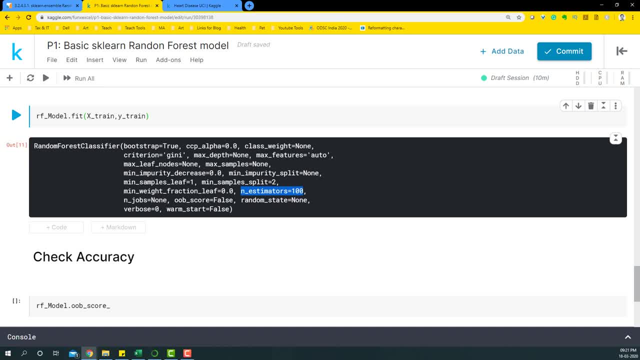 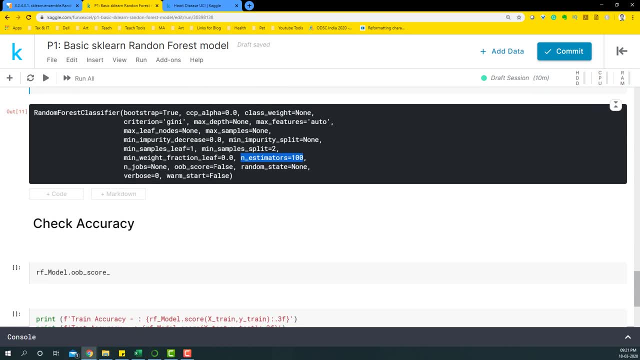 with hyperparameter tuning right. so for now we're just going to focus on building the basic model and see how the accuracy looks like generally when we do a random forest, there is a oob score that is available in this particular model. since it's false, we're not going to be looking at that. 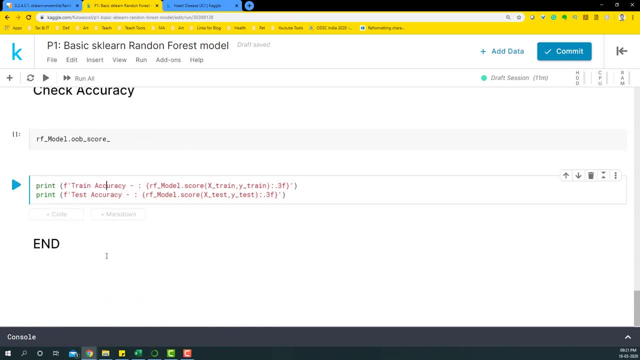 particular score, we're just going to be looking at the accuracy of it. so if i run this particular accuracy here, you'll see that the train accuracy is one which means random forest has overfitted this training data, which means that it's not going to be doing good on the test data set. and 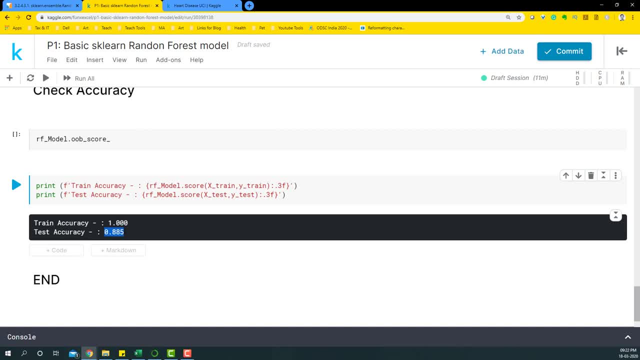 like i said, you know, the test accuracy is around 0.885, which is a big difference to the train accuracy that we have here. essentially random forest: yes, it does good, but it's also known for overfitting the model. to really fit a good random forest model, what we need to do is we need to. 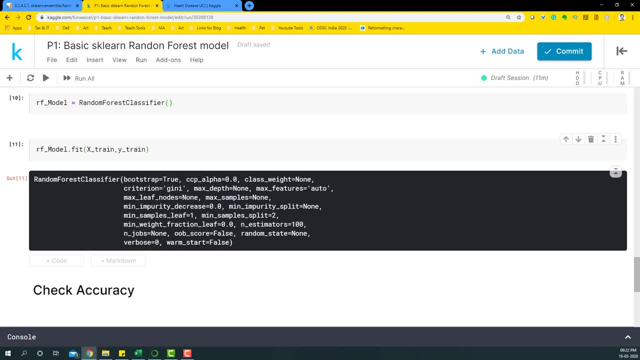 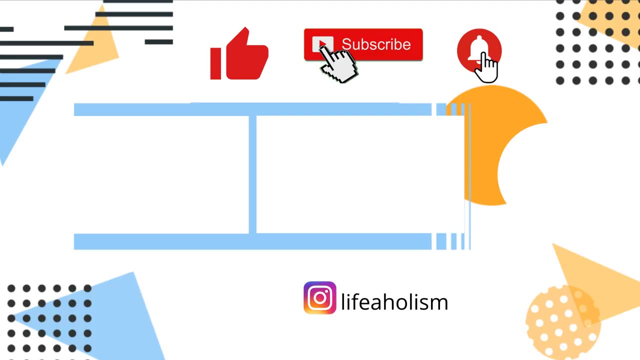 do is use the hyperparameters and grid search to identify a good model that will also have a good test accuracy, along with the train accuracy, right? basically, it's balancing the bias and variance to build a good model. so our next video we're going to be doing random forest. 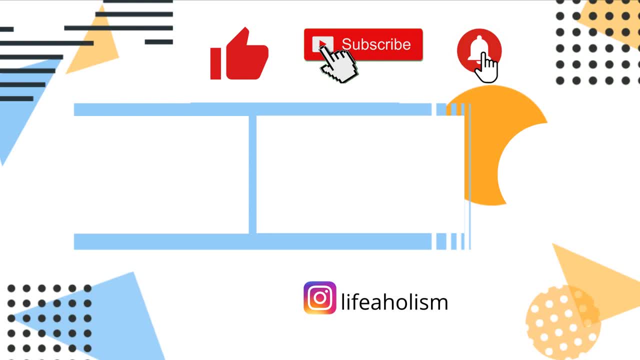 hyperparameters tuning. thank you for watching this video, guys. if you like this video, please hit the thumbs up button and please don't forget to subscribe to my channel.